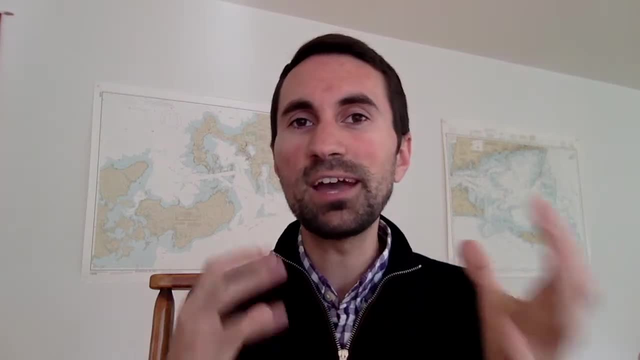 about each model. If you watch them long enough, you'll see very, very good results, and there are nothing wrong with those. I'll go to some more responses instead of my own assessment. Watch the video and determine which one drew the most data, and I'll see which one casted. 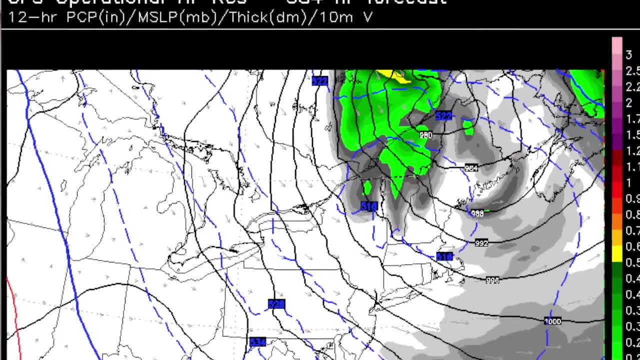 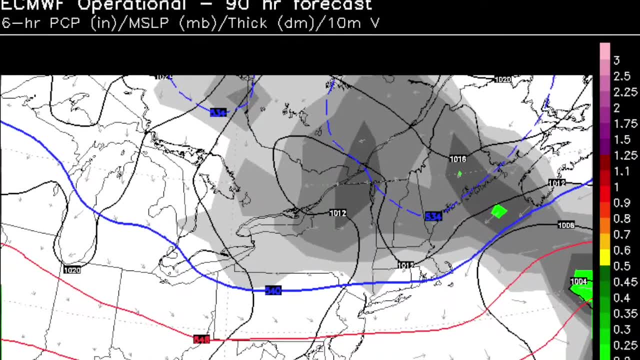 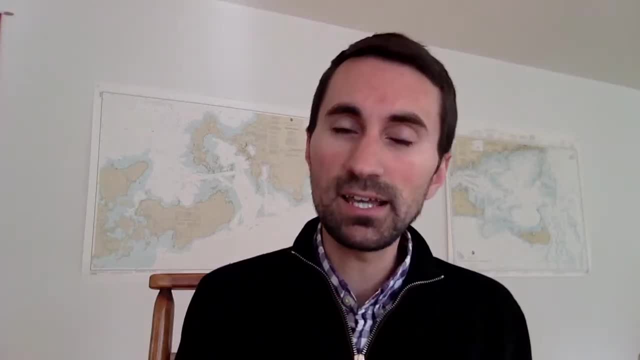 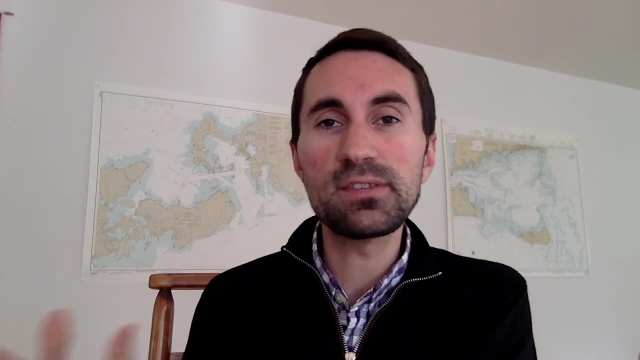 So this is a flew- 너무 실� really, Bohr Kapitscher. why that is has to do with funding. Basically, in Europe, you have to pay for the data that you get from this model, so there's more money going into its. 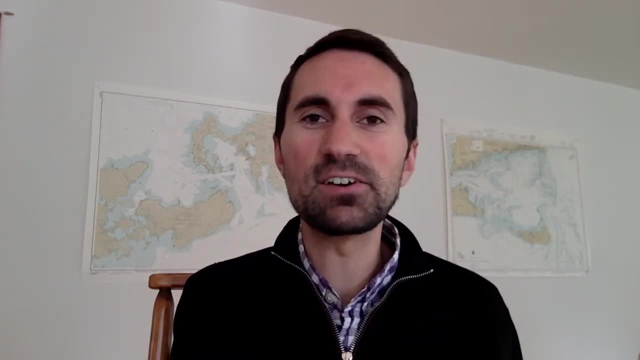 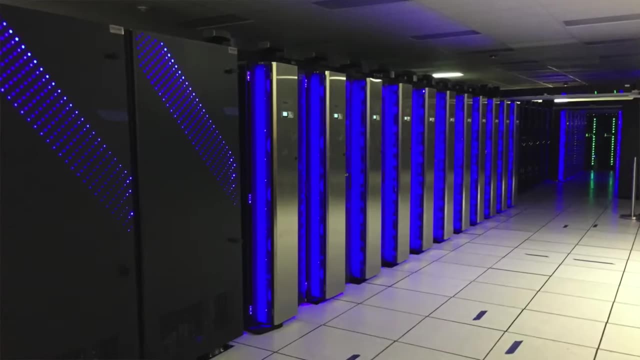 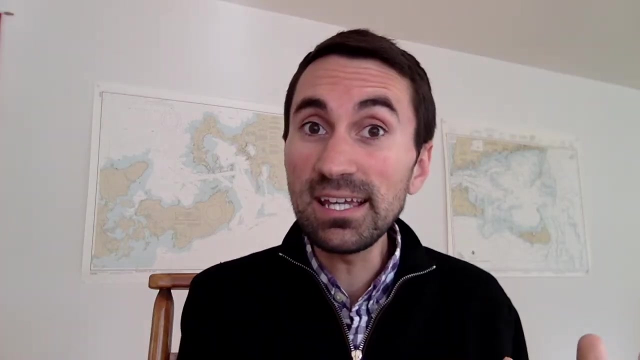 continued development. Meanwhile, on this side of the Atlantic Ocean, the GFS is taxpayer funded, So you're reliant upon government funds to build up the computing power, And it is getting better. that's the good news. More money is going into it, but because it's free and taxpayer funded, it doesn't have the same 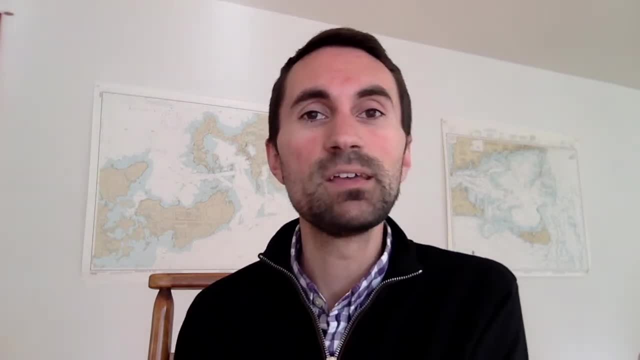 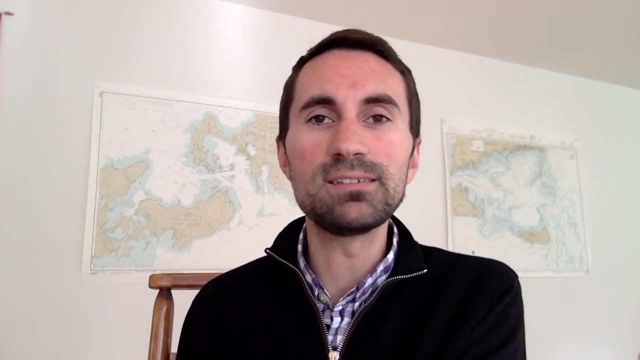 resources that the European has. It's really just that simple. The European model is definitely still the benchmark model to look at. Doesn't mean it's always right, but it means it's more often than not going to give you a better sense than another model might. There are another type of model here. 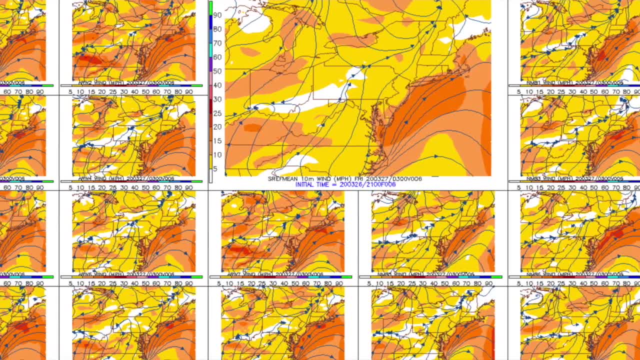 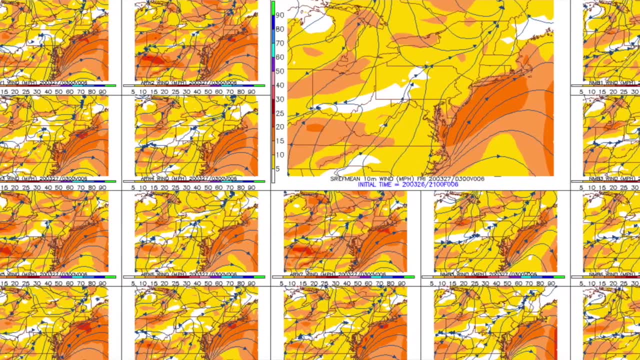 that we look at. they're called ensembles. Basically, these are models that take the starting point in the atmosphere and they'll tweak the atmosphere. They'll tweak the atmosphere and they'll tweak the temperature One or two things. So let's say, the temperature right now is 52. One. 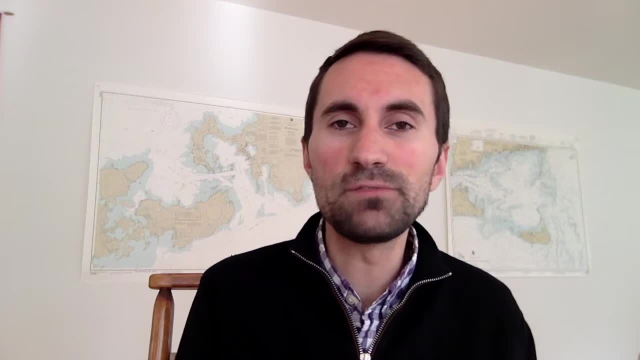 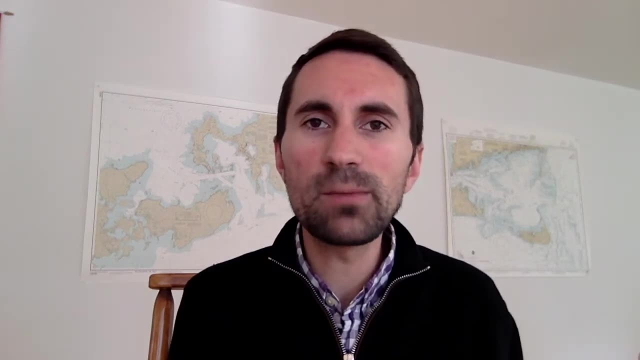 model will change that and make the current temperature 51. Another will make it 53,, maybe 55, maybe add more clouds to what's happening now, Basically tweaking the environment right now, assuming that we're never fully able to get a great. 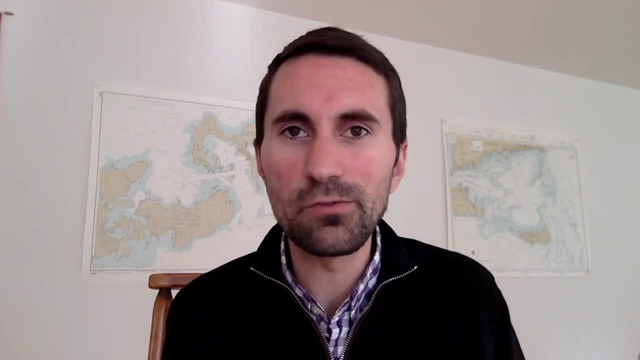 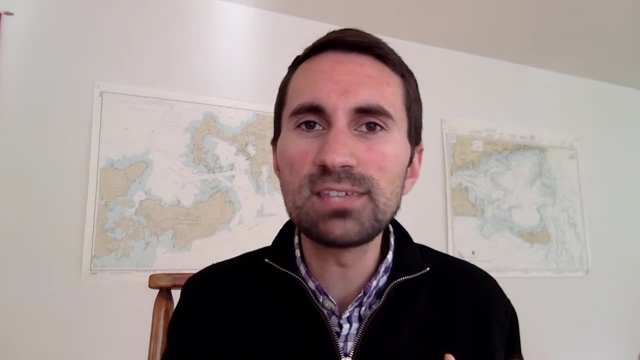 picture of what's happening even now, because we don't have observations all over the world. There are obviously gaps, our measurements might be off a little bit. so you tweak these starting variables and then use them to say to the model: okay, let it rip. And then you see how each model plays. 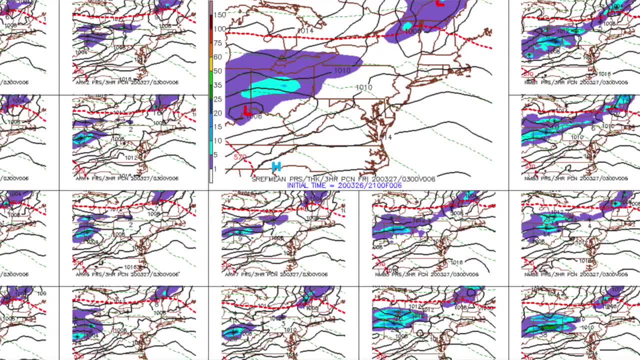 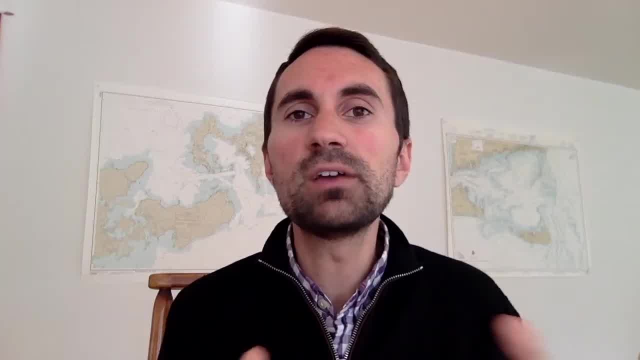 out. Each one will be a little bit different because you tweak those starting variables. These are ensembles and you can run 25, 50 of these- even more in some cases- and then you get an average, And that's usually a good way to.